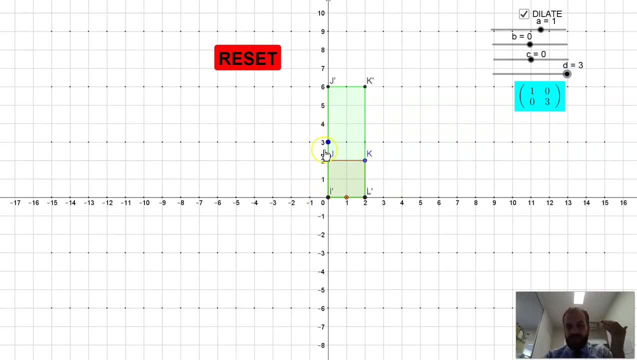 to 3. you can see that I've stretched away from the x-axis and that point which was 0- 1 has now been moved up to 0- 3 and all points have been moved by that factor of 3.. So the point that 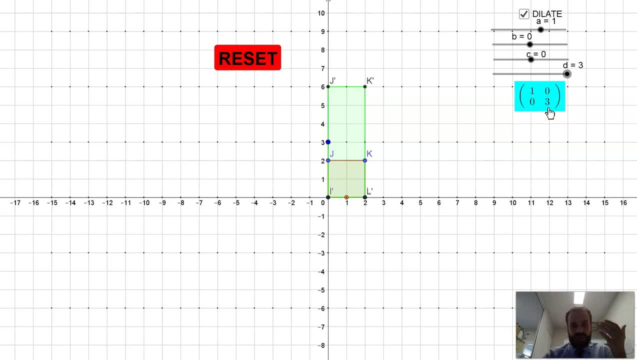 was originally 0, 2 is now 0, 6, and obviously we can take it back the other way And of course we can do both of these things. So we can do a squash and we can do a stretch, and we've transformed our 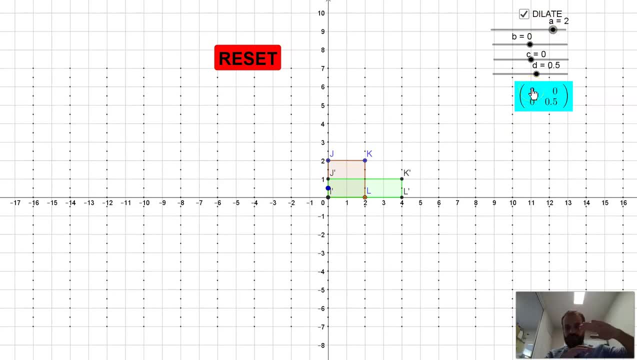 matrix by squashing it and stretching it, dilating it in both directions, by changing where our x coordinate our 1: 0 goes and where our y coordinate our 0: 1 goes. Let's put it back how we found it. that's really all I want to talk about graphically there. Now let's take a look at some sort of meaty. 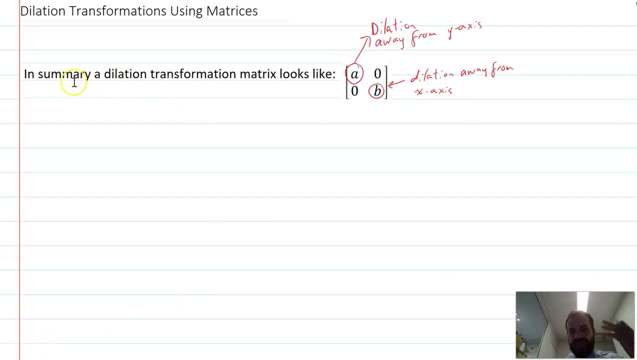 algebraic questions. So this is kind of the note I need to take. In summary, our dilation transformation matrix looks like a 0, 0 b, where a stretches away from the y-axis and b stretches away from the x-axis, And this image is probably a good example of that. Let's call this a 2 by 2 square. So 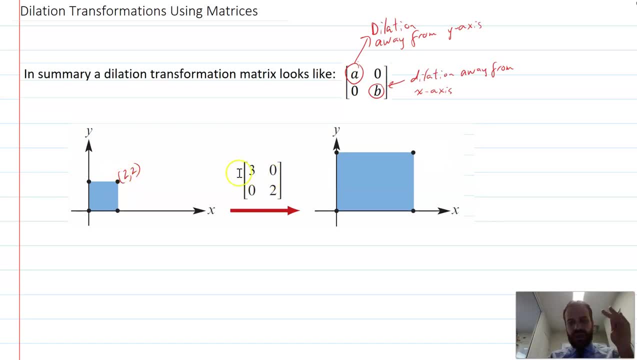 all right, so there's our 2 by 2 square. Now what's going to happen to our 2 by 2 square if we use transformation matrix? Well, that 3 is going to dilate it away from the y-axis, So that 2, that x. 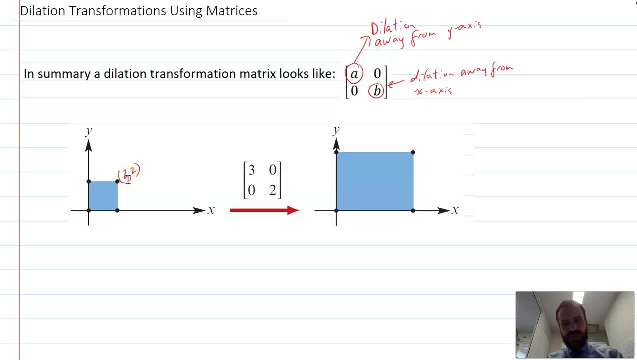 coordinate is not going to be 2 anymore, It's going to be 2 times 3.. So it's going to be 6.. So 3 times wider. And that 2 here. the y, this b value here, dilates away from the x-axis, So it's 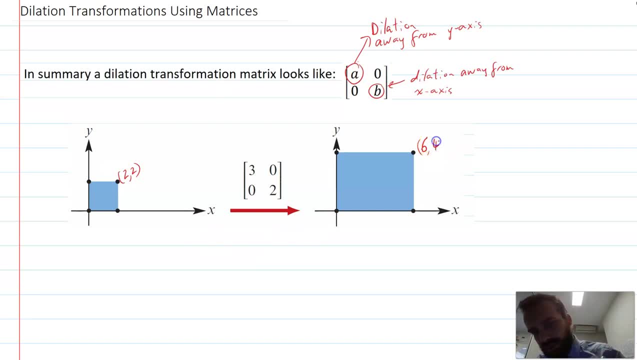 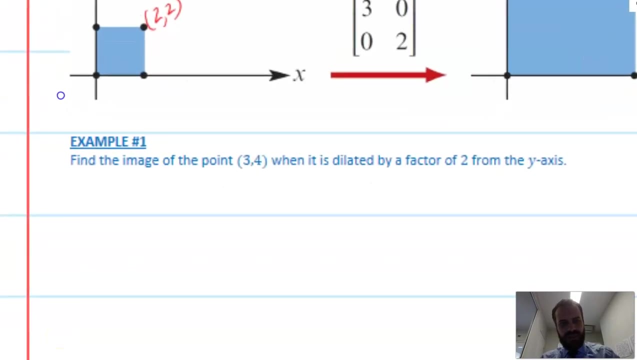 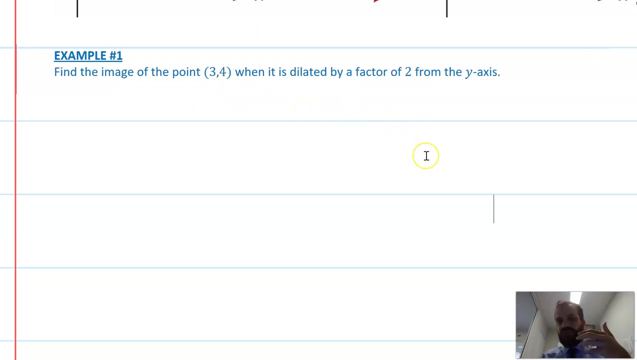 not going to be 2 anymore, It's going to be 4.. All right, so that's a another sort of graphical look at what these dilation transformation matrices do. All right, that's that done. Let's jump into an example here. Find the image of the point 3- 4 when it is dilated by a factor of 2 from the y-axis. 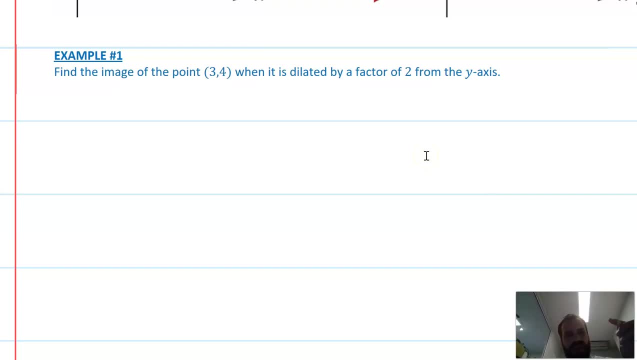 Okay. so what do we want? We want the image of the point. Let's call it point a. So the image of the point a is going to be a dash, And we can say that a dash is going to be equal to the linear transformation matrix times a. Okay so. 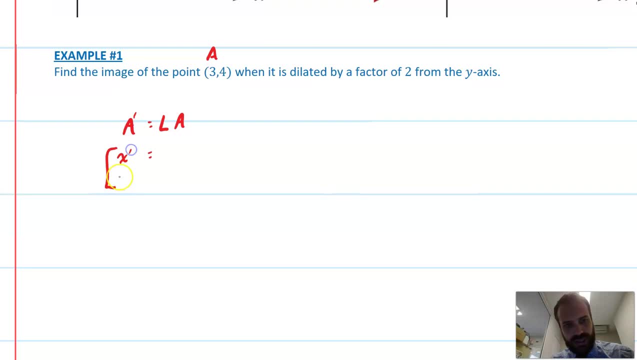 a dash. we can just call it x dash, y dash. The linear transformation matrix is going to be a 2 by 2 matrix, And a is the point that we're interested in, So we're going to call it x dash, y dash. 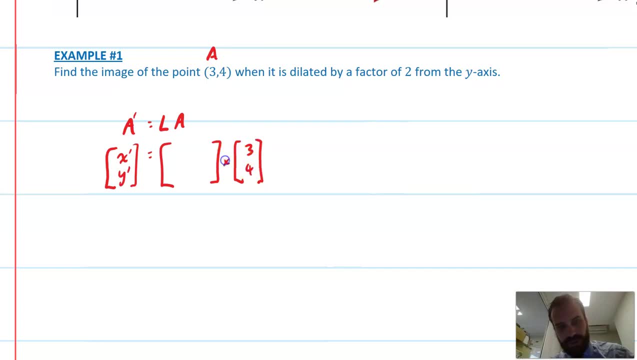 We're interested in 3, 4.. Okay, now, what's the linear transformation matrix? Well, there's going to be zeros here and here. Now, when it is dilated by a factor of 2 from the y-axis. So I'm stretching away from the y-axis, So that's going to affect my x-coordinate, It's going to move my x-coordinate. 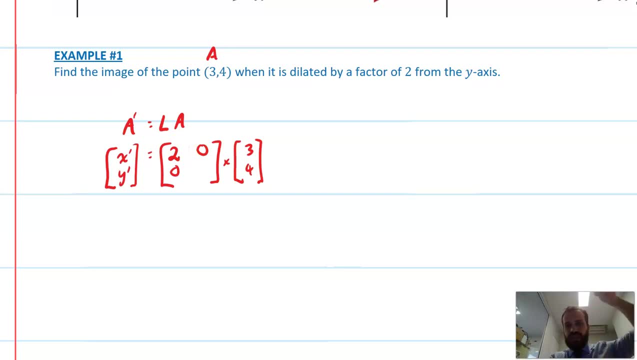 up by a factor of 2. It's not stretching away from the x-axis, So that x-axis remains unaffected From here. it's just basic matrix multiplication And you can do that. But it's 2 times 3 plus 0 times 4. Which will be 6. And it's 0 times 3. 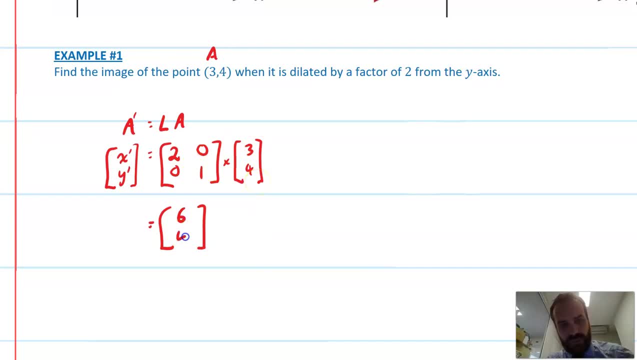 plus 1 times 4.. Which is 4.. Now, stop and think about that for a minute. Does that make sense? Well, find the image of the point 3, 4, when it is dilated by a factor of 2.. From the y-axis, it's now 6, 4.. Yep, that makes sense. It's dilated a factor You probably could. 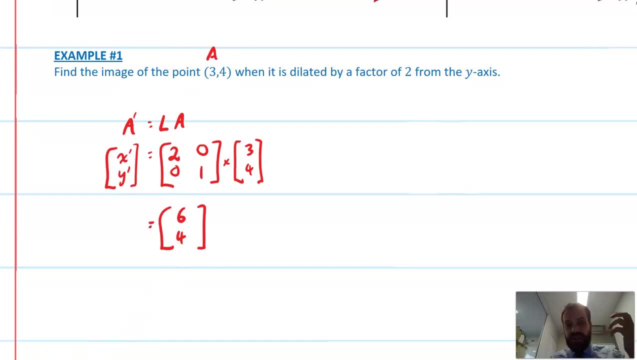 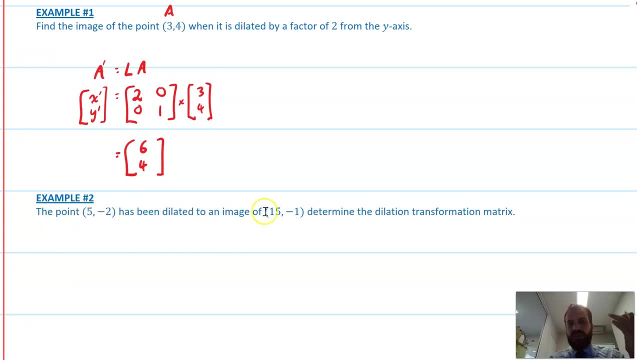 have done this without matrices, But obviously we're going to do more tricky stuff in the near future. All right, and come to our second one here. The point 5, negative 2 has been dilated to an image of 15 negative 1.. Determine the dilation transformation matrix. Now this feels very. 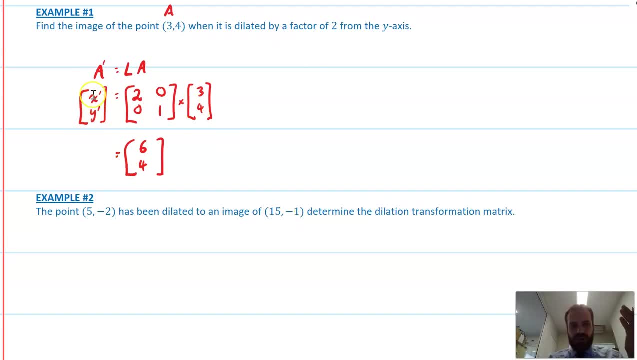 similar to this one, Except this time we know the image, We know the original. What we're missing is the linear transformation matrix, So let's start working on it and see where we end up. The point 5, negative 2.. Well, that's the original original point. 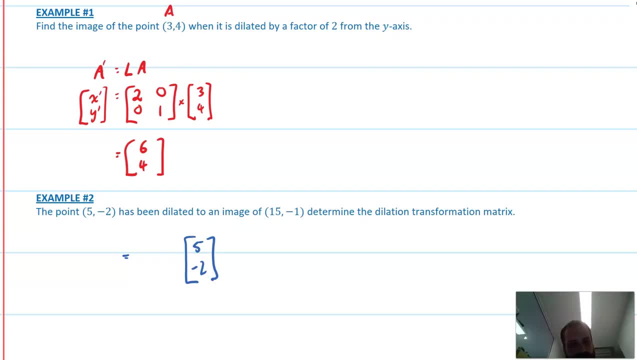 Has been dilated to an image of 15 negative 1.. That's the image. Determine the dilation transformation matrix. Now we know it's going to be like 0- 0. 0 here and we know that we're going to have an a, b there. Now there are different things you can. 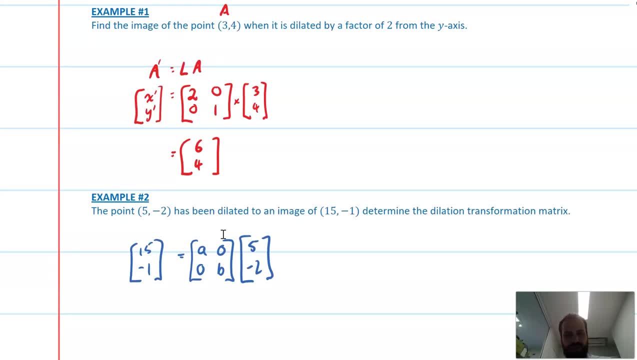 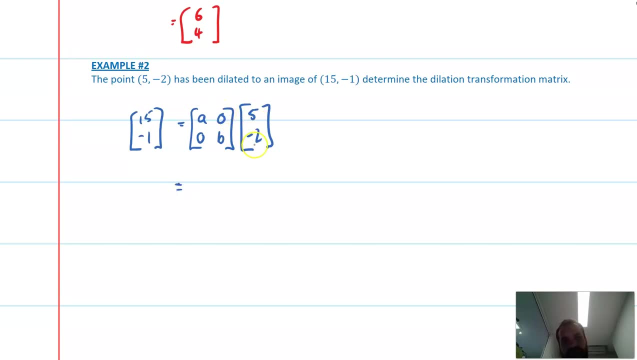 do here. But the easiest way forward is now to just multiply through and you'll see what happens next. We get a times 5, 0 times negative 2.. So that's just going to be 5 a, And we get 0 times 5 b times negative 2.. That's going to be negative 2 b, And we can now. 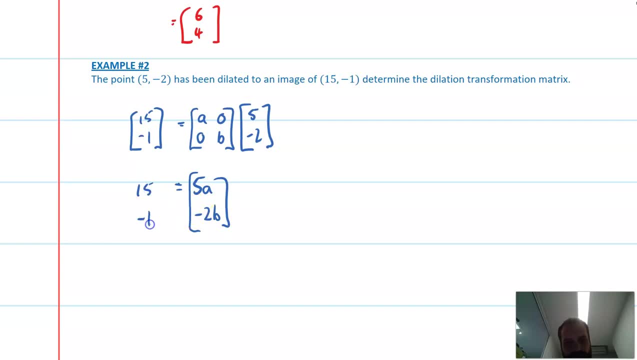 say that 5 a negative, 2 b, 15 negative, 1. And now we can just solve those elements Because we're saying this matrix is equal to that matrix, So that element must be equal to that element And that element must be equal to that element. So therefore, 15 equals 5 a And a equals 3.. And 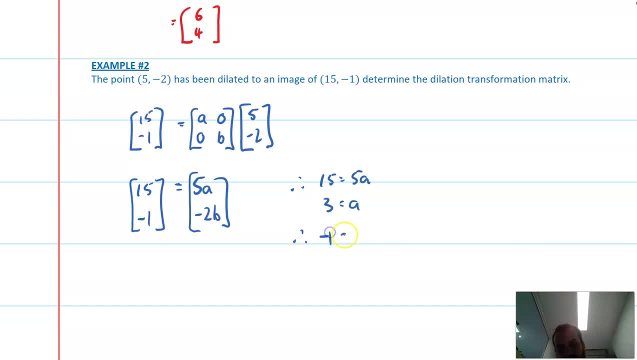 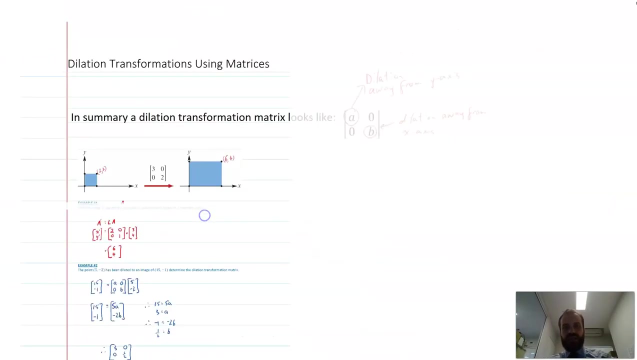 therefore, negative 1 equals negative 2 b And b equals one half. So the thing that we were trying to find, It was the dilation transformation matrix. Therefore, it is 3: 0, 0, 1 half. Okay, That is dilation transformation. 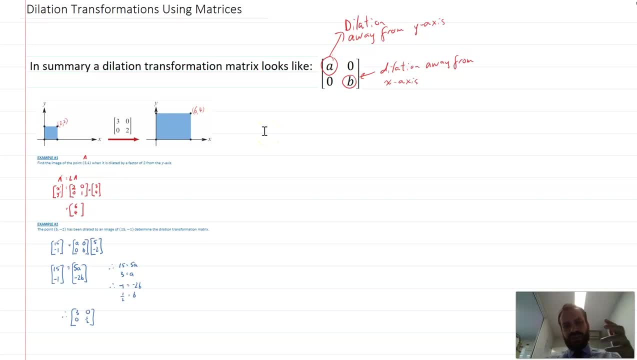 using matrices. And just before we go, this video done, I do want to sort of show you some notation here. It's not as useful for the dilation stuff, but you might get asked to display it this way, but it does get more useful as we. 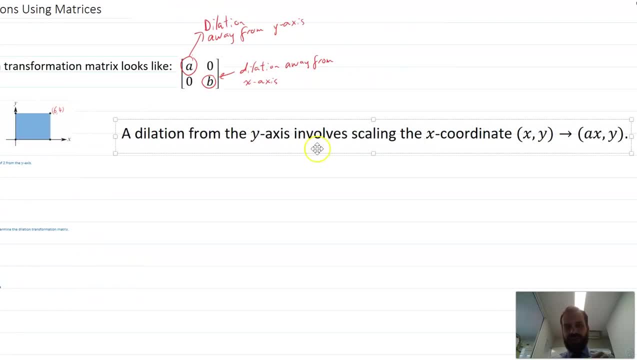 move through. So here's our first little bit. A dilation from the y-axis involves scaling the x-coordinate xy to axy. So whatever that a value is in our matrix, that's what you multiply your x-coordinate by when you do that dilation. Now, obviously there's a second version of this one. 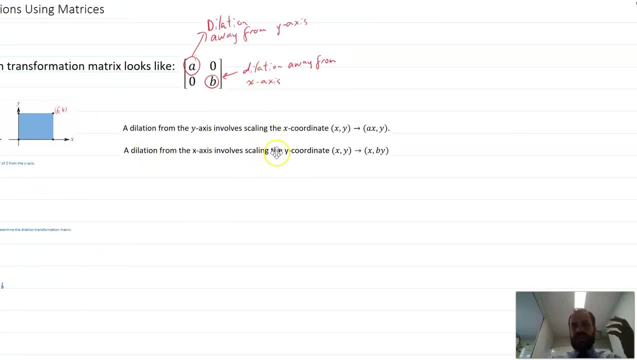 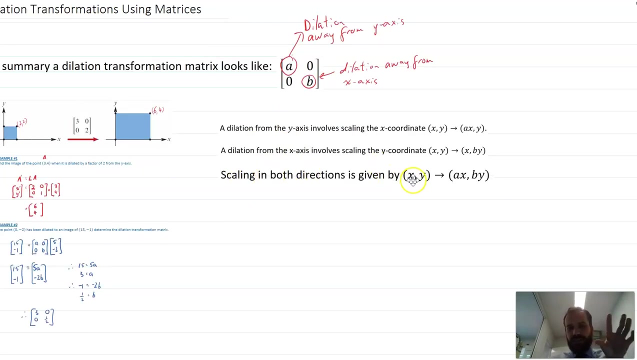 a dilation from the x-axis. So stretching up involves scaling the y-coordinate by going from xy to xby whatever that b value is. Now, of course, we can combine these two into one. Scaling in both directions from the point xy gives you the image axy. 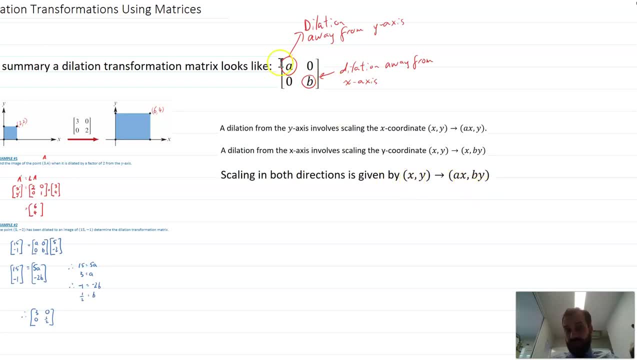 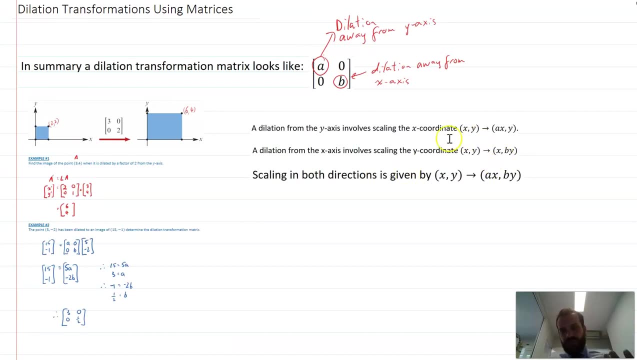 x, b, y. Multiply the x-coordinate by a, multiply the y-coordinate by b. Pretty straightforward stuff. but when we start moving into the more complicated transformations, being able to work with that kind of notation is going to make your life a lot easier. 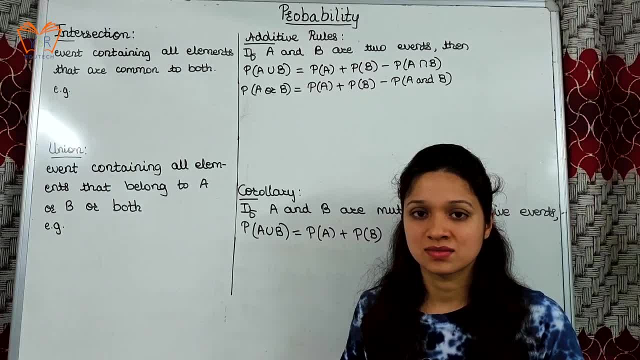 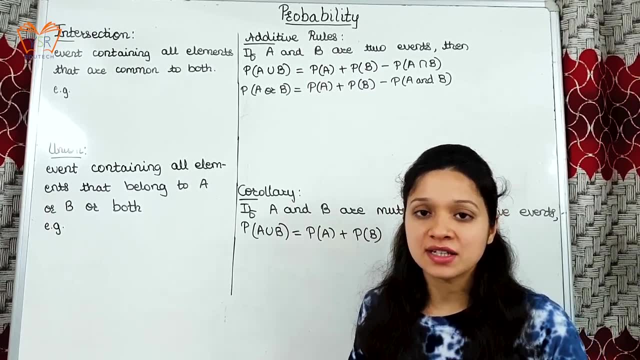 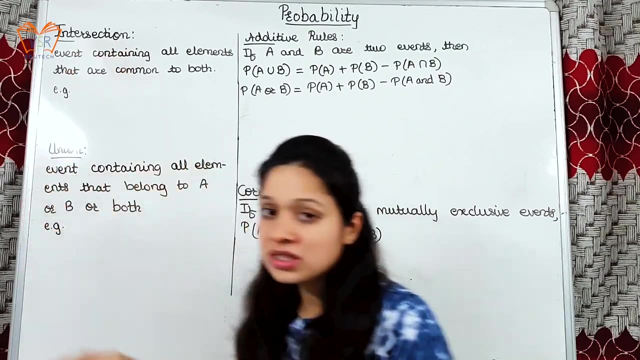 Hi guys, I'm Suprabha. In the first video we studied all the basics of probability and then in second video we studied what are events and different types of events. In this video we'll move on to the terms called intersection, union and additive rules. Additive rules are: 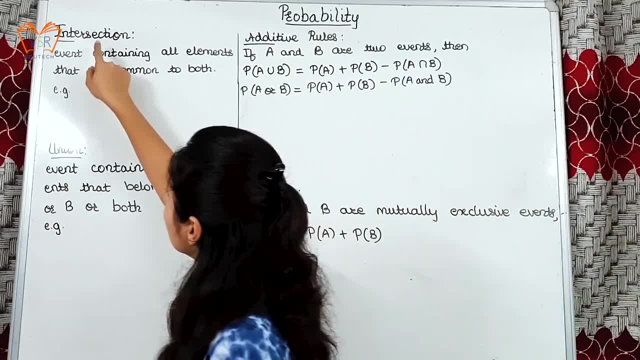 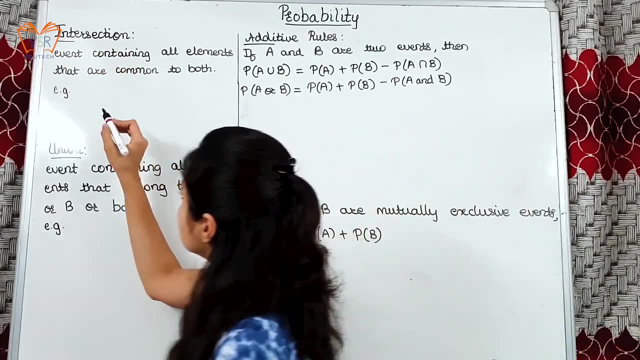 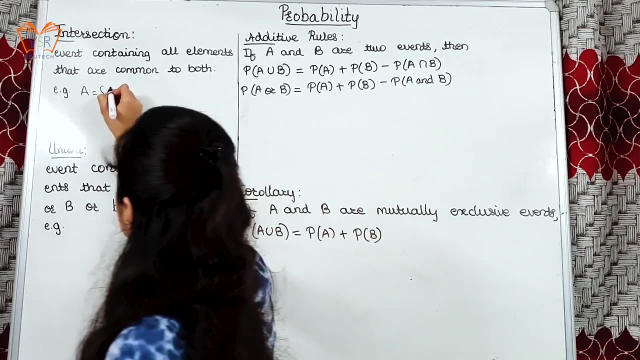 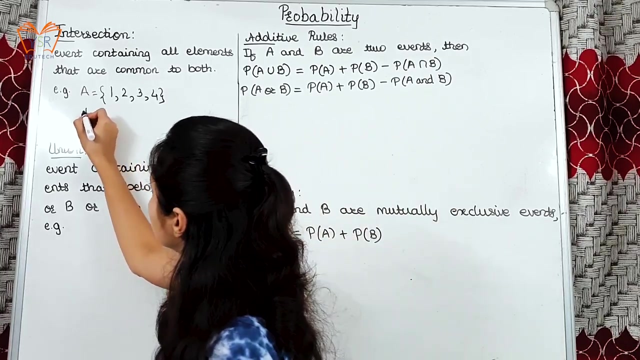 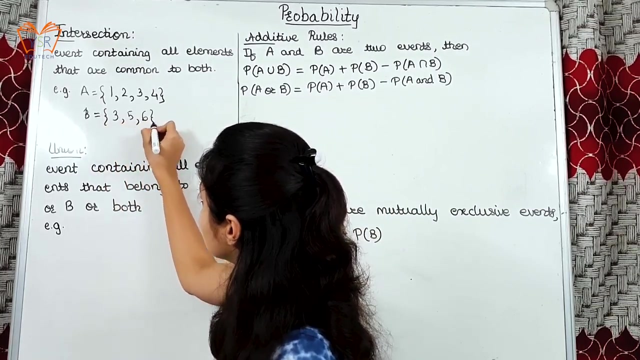 the addition rule for probability Intersection event containing all the elements that are common to both the events. This simply means, suppose there is an event A that consists of elements 1,, 2,, 3, 4, and then we have event B. It consists of elements 3,, 5, 6, and we are supposed to find: 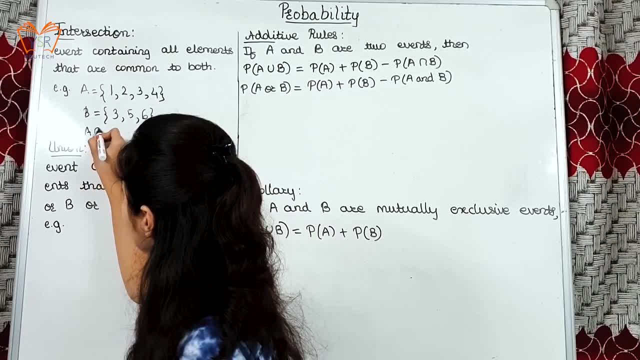 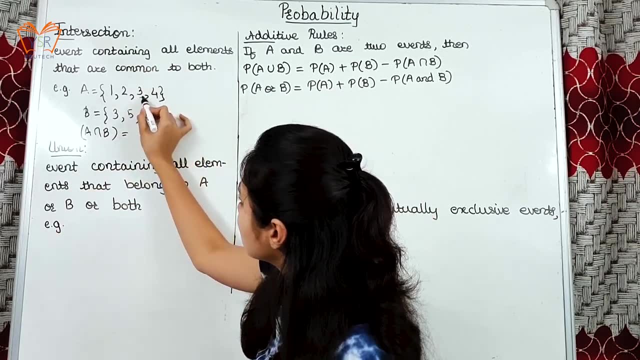 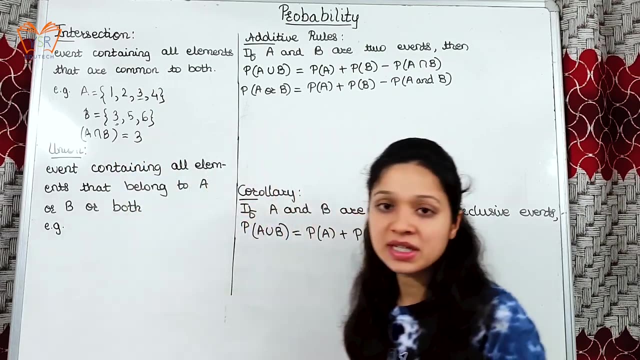 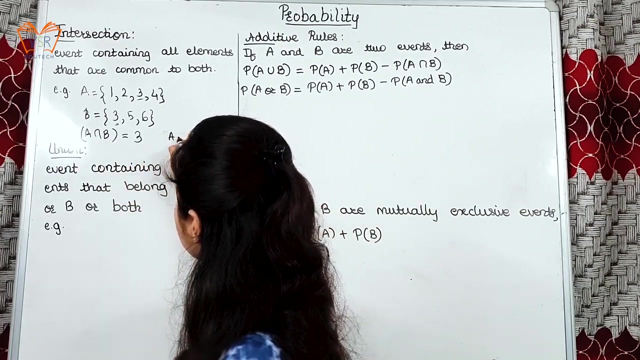 out the intersection of A and B Elements common in both. You can see there is only one element that is common, So intersection of A and B will be one element, that is, 3.. This is also written as A and B. This intersection. 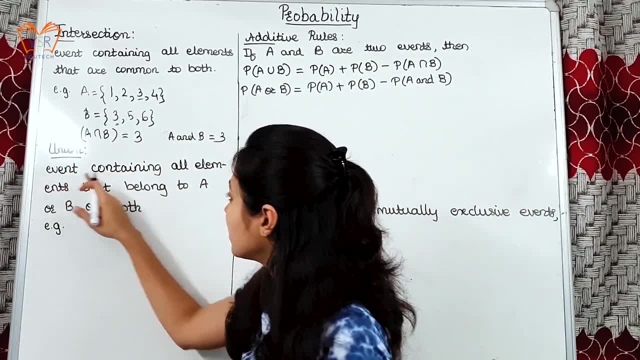 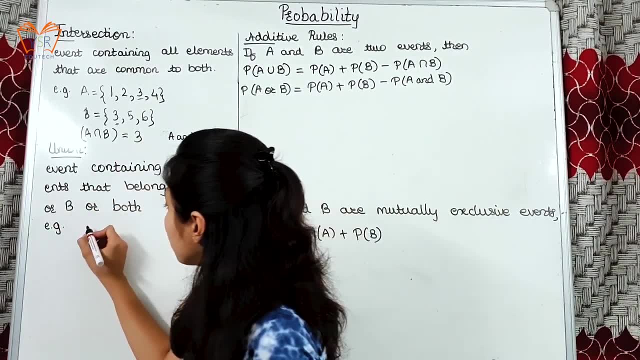 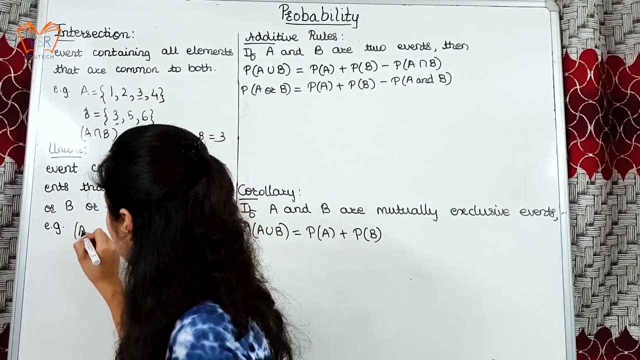 only means and Union Containing all elements that belong to A or B or both. We'll take the same example: Element A with these elements, B with elements 3, 5, 6.. So A union, B, It says all the elements.